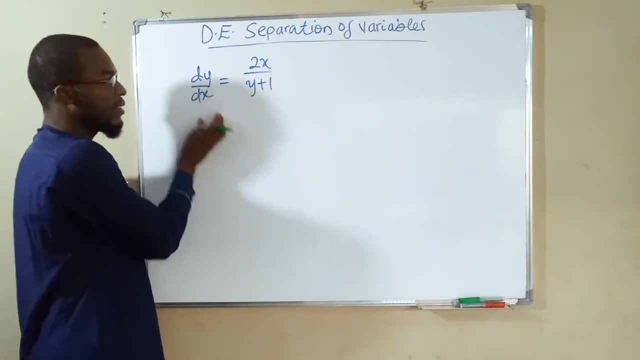 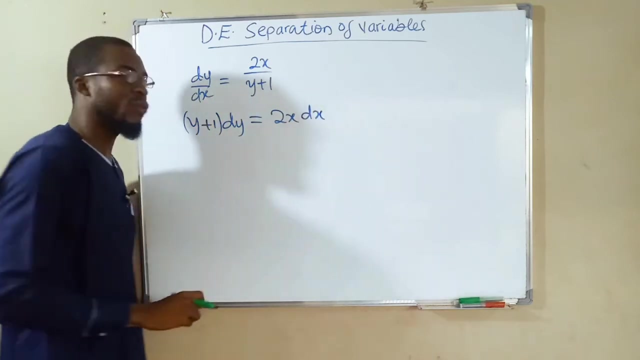 we have to separate these variables. Now we are going to take dx to the right hand side and bring y plus 1 to the left hand side, So we have y plus 1 dy. If it comes to this side, this is equal to 2x. then dx. if dx go to the right hand side. 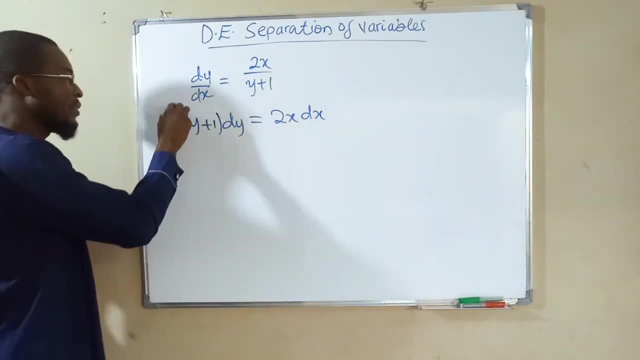 So now we are free to integrate this equation. We integrated the side. we also have to integrate the other side, So we are going to integrate this independently. for why we have y squared over 2 plus, if you integrate 1 with respect to y, you're going to have: 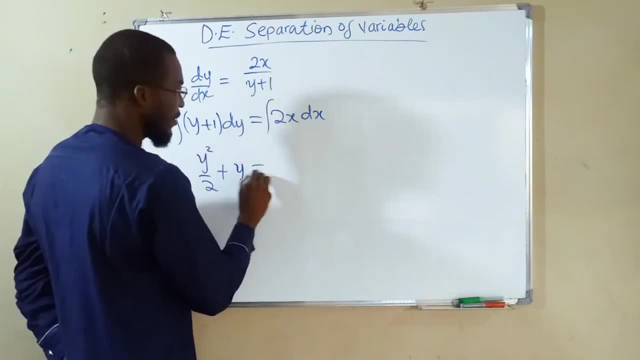 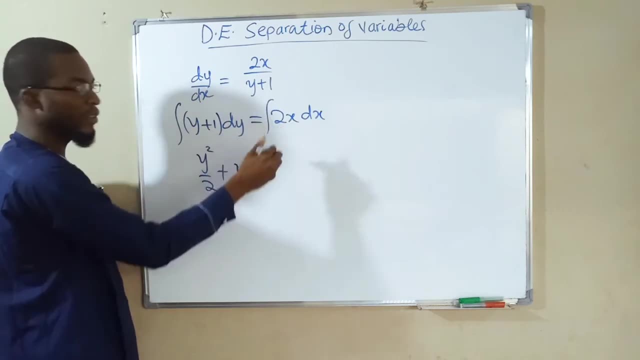 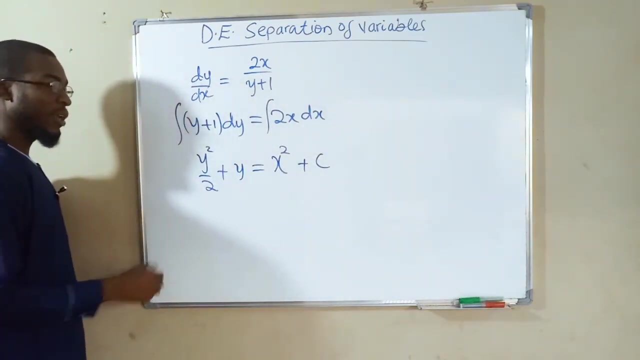 10, just Y. and to the other side. you know, the power of X will increase by 1, which is going to be 2. then, divided by 2, 2 will cancel, to leaving only X squared plus our constant of integration. you can multiply each time by 2 in order to. 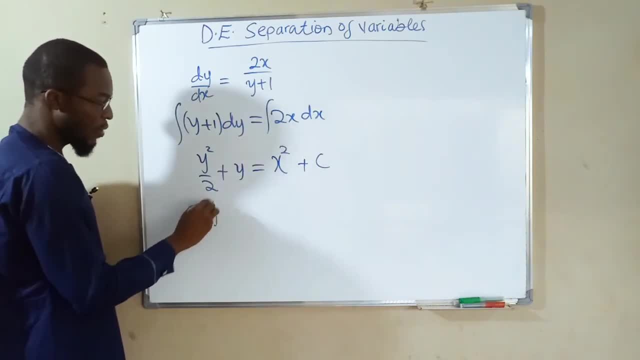 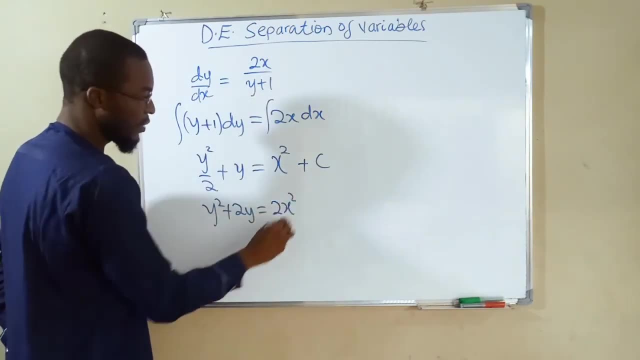 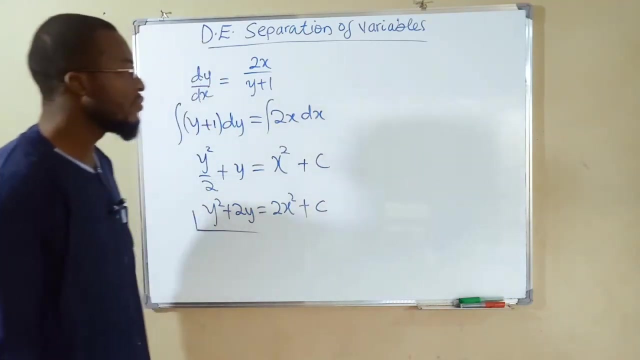 clear the fraction so that we have Y squared plus 2. Y equals 2 X squared plus 2 C. but multiplying constant with constant is still constant, so we have C. so this is our general solution for this differential equation. now let us look on to another one. here is our next question. 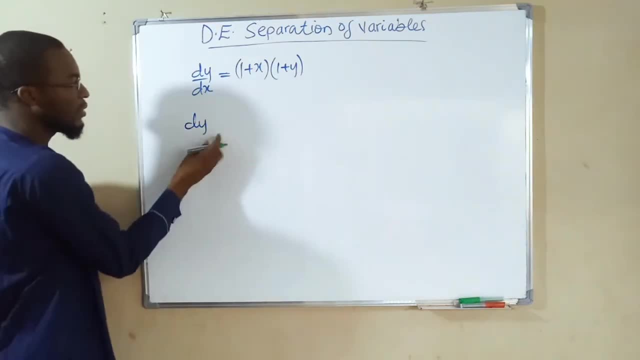 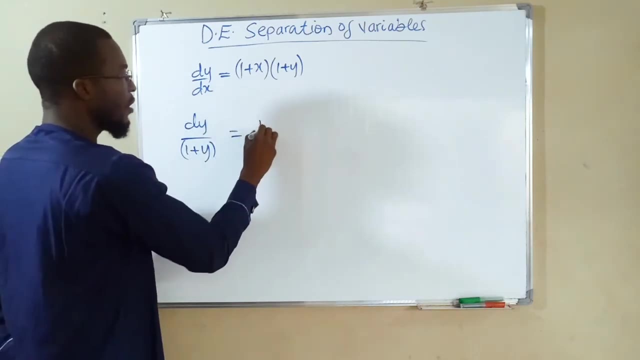 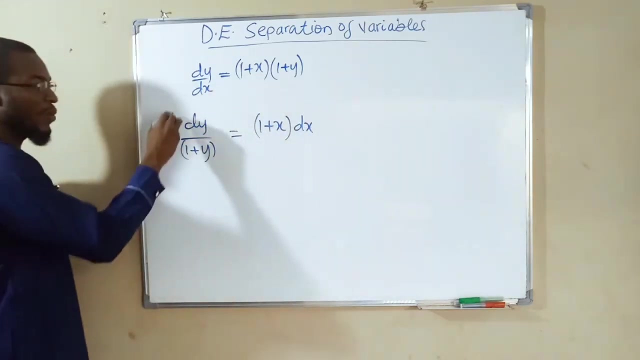 dy. then we bring this one backward over 1 plus Y and this is equal to 1 plus X. then we take DX to the right hand side. we have DX now we integrate both sides of this equation. if you integrate this, you are going to obtain the natural log. 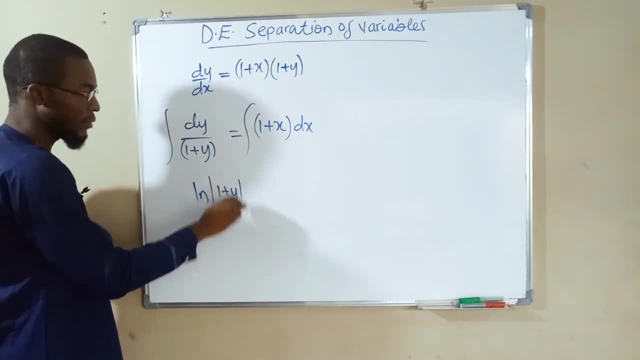 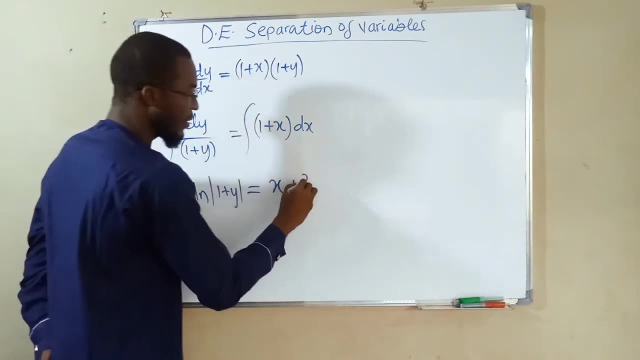 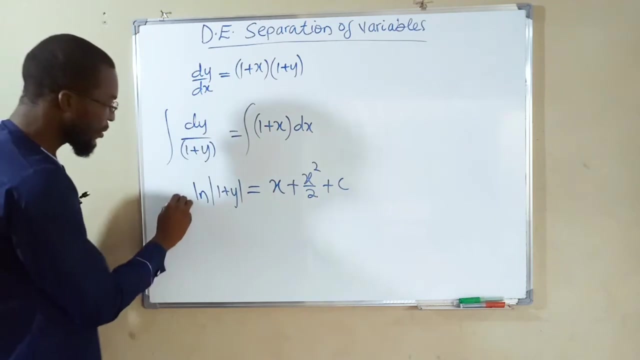 of the absolute value of 1 plus Y, and to the right hand side we have this equal to X, and this equals to x squared over 2 plus the constant of integration. So this is the general solution for this differential equation. Let's look on to another one. 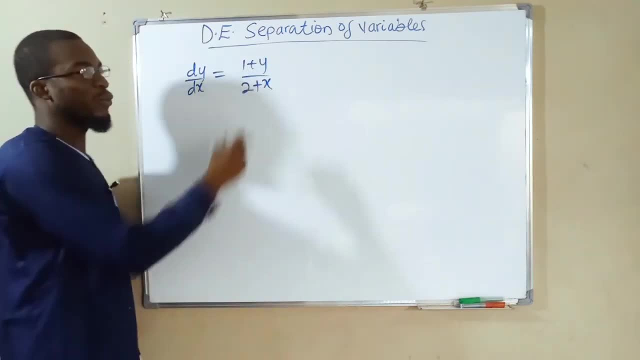 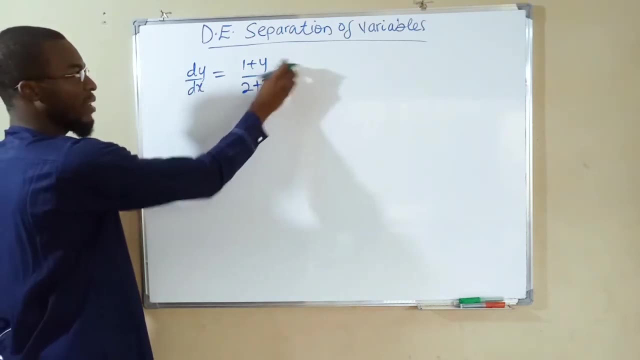 This is another question. Now we have dy over dx, equal to 1 plus y over 2 plus x. To separate these variables, we are going to take dx to the right-hand side and bring 1 plus y to the left-hand side. 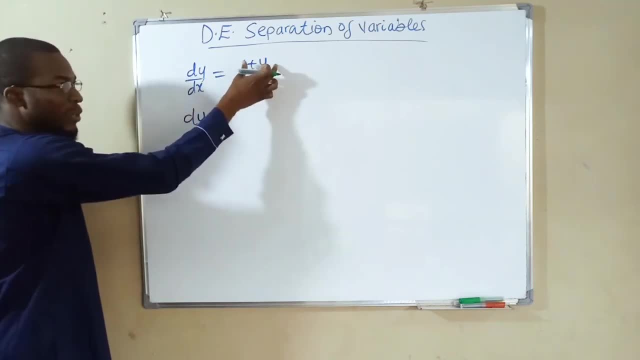 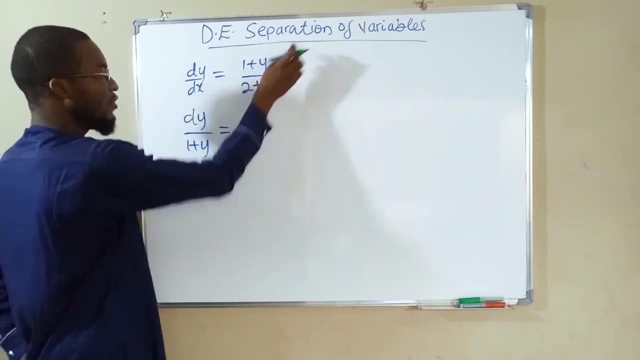 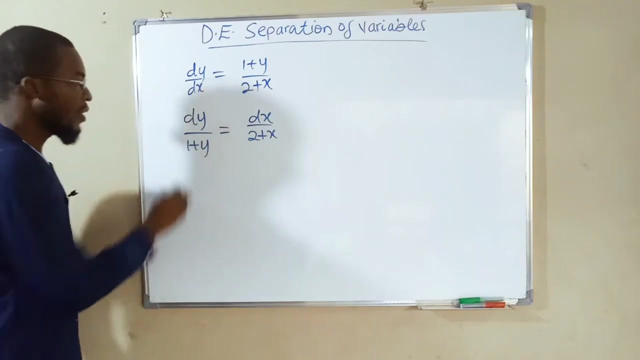 So we have dy. If you bring this one backward, it becomes 1 plus y. This is equal to you. take this one to the right-hand side: it becomes dx over 2 plus x. Now we are going to integrate both sides of this equation. 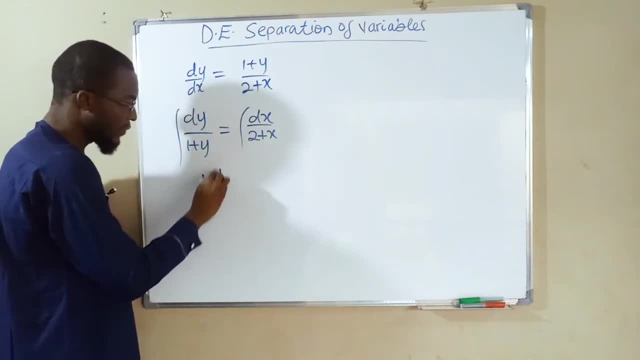 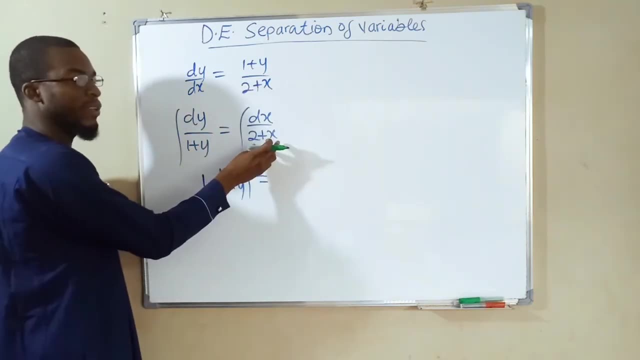 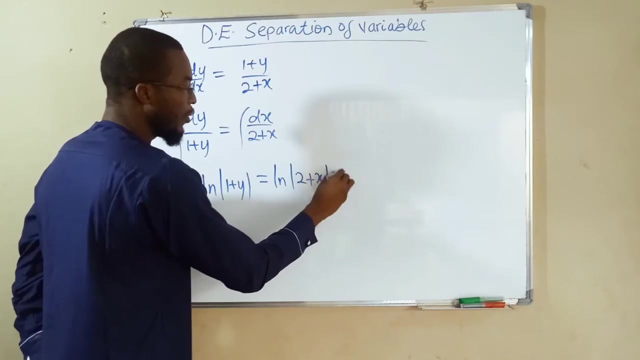 If you integrate this, you are going to obtain the natural log of the absolute value of 1 plus y. This is equal to. Again. if you integrate this, you are going to obtain natural log of absolute value of 2 plus x, plus the constant of integration. 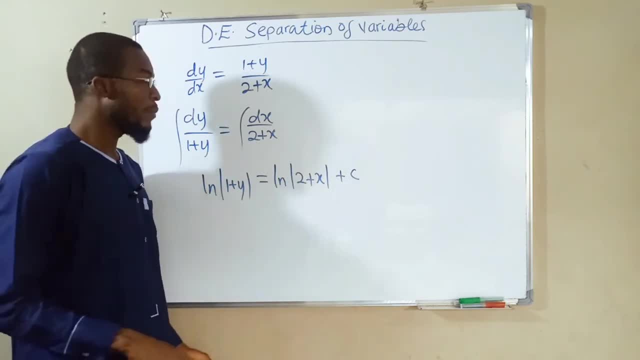 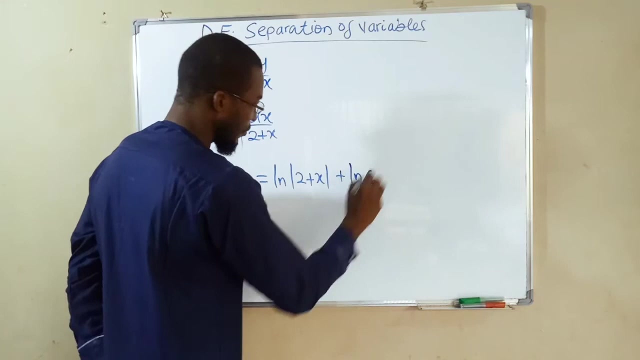 Having a natural log in an equation is not a problem because so many natural logs can be differentiated. But to get rid of this natural log you can even take the natural log of c for convenience. So we have lnc, So that natural log of 1 plus y. 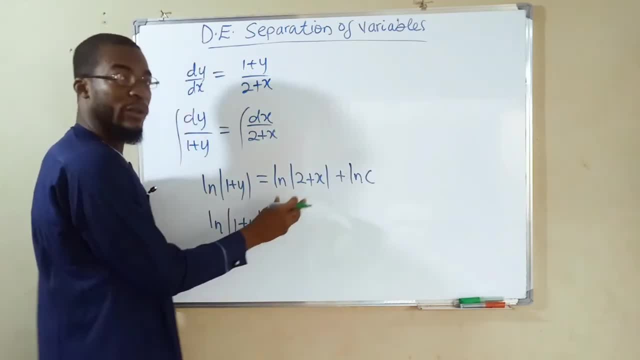 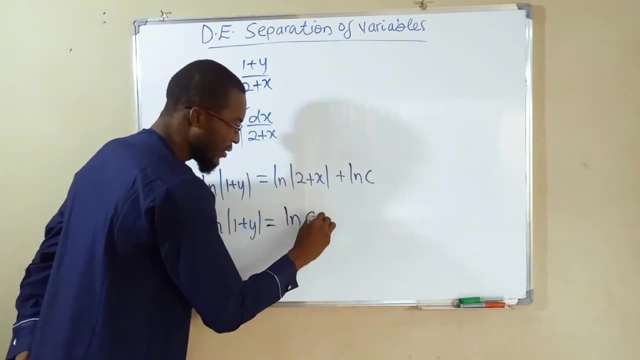 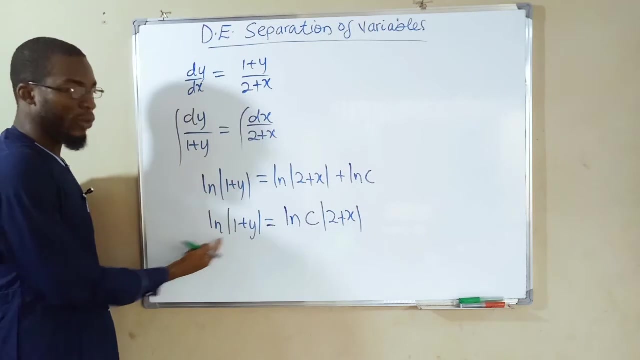 will now be equal to Using laws of logarithm. you can transform these two terms to have a single log. This is equal to the natural log of c. absolute value of 2 plus x, Since we have common log to both sides. 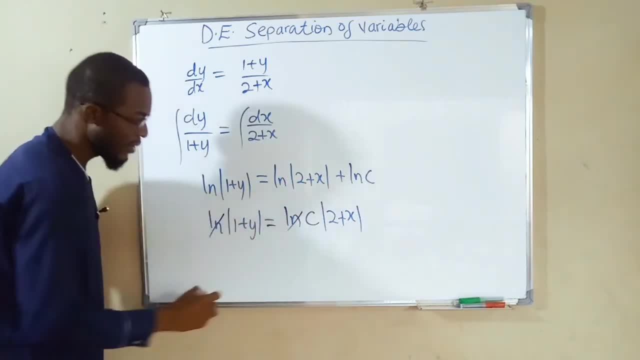 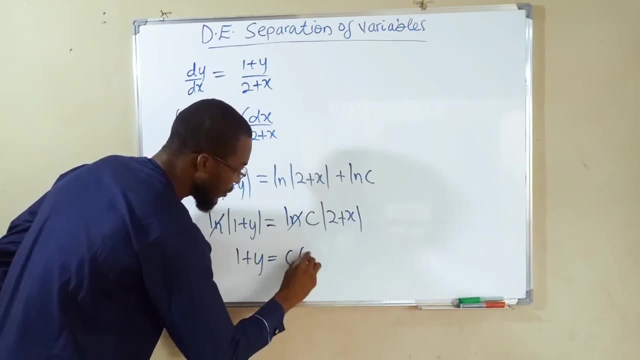 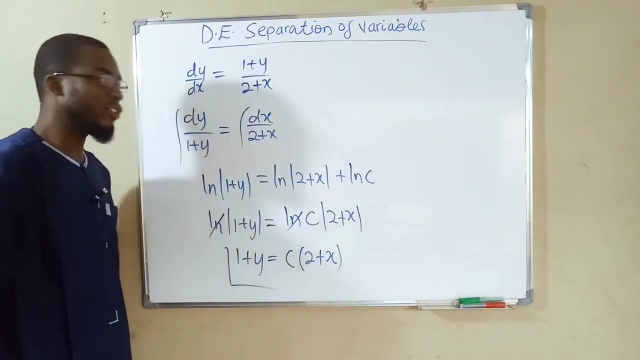 we can cancel each. So we have this, cancel this. Finally, we have 1 plus y, which equals c times 2 plus x. Therefore, we say this is the general solution for this differential equation. And this is our next problem. 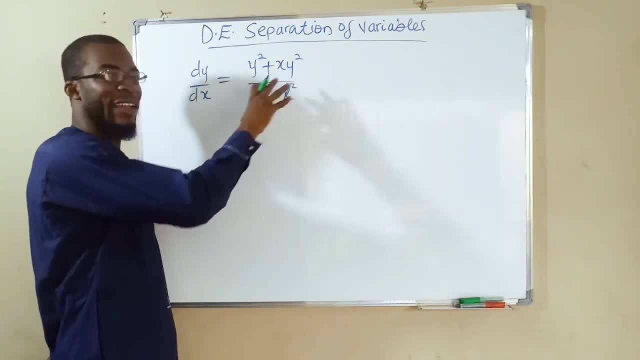 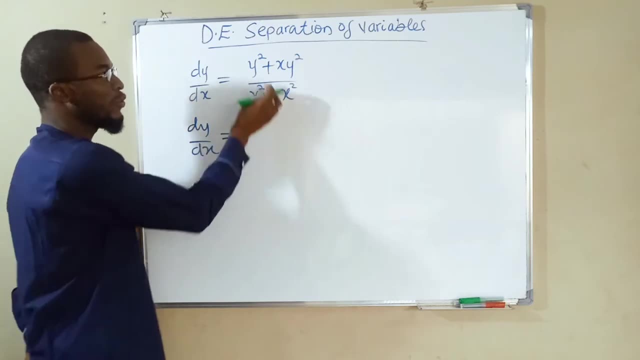 But if you look at these functions, they are entirely mixed up. So let us factorize them. So we have dy over dx And this is equal to. From these two terms, we have y squared in common. We have y squared. 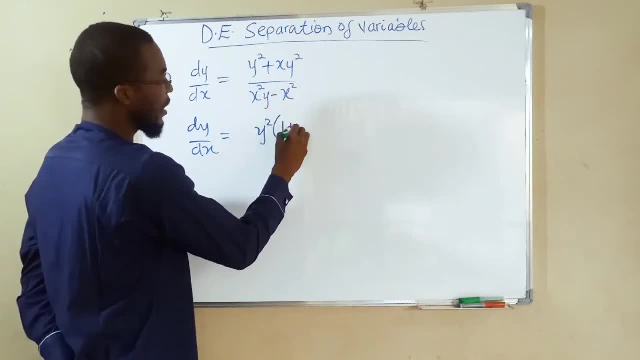 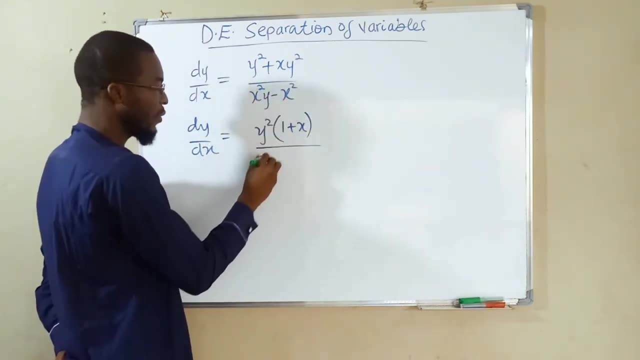 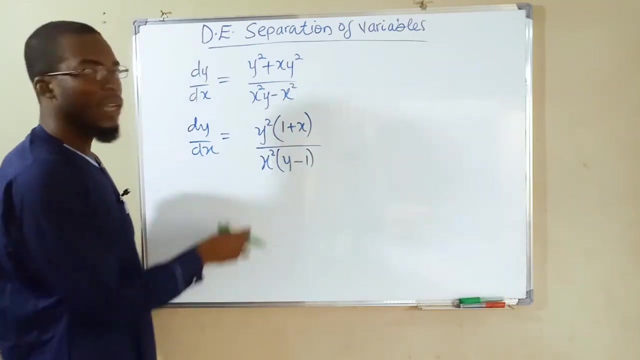 We have y squared in common, But inside we have 1 plus x. On the denominator we have x squared in common. So we have x squared In bracket. we have y minus 1.. Now we want to separate the variables. 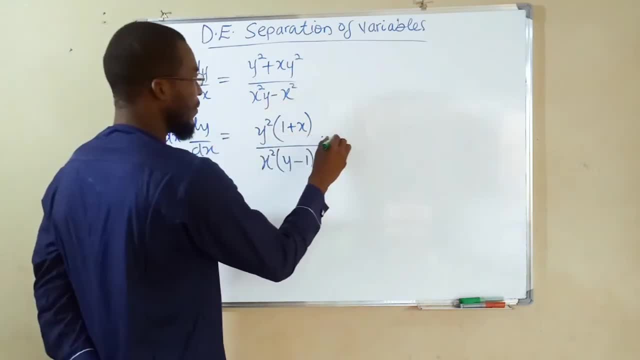 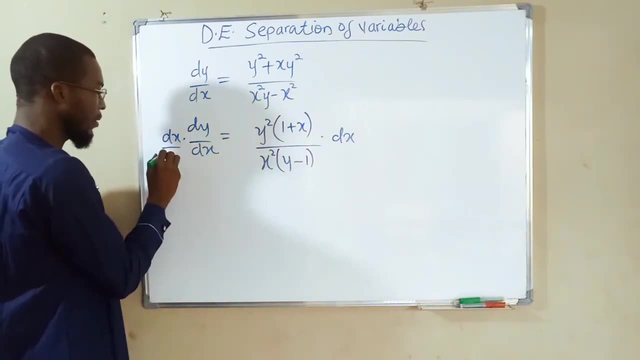 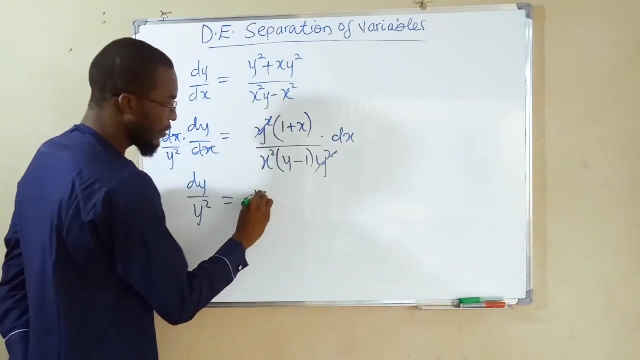 Let me multiply dx first. We have dx. Let me divide by y squared, So we have y squared. We have y squared, So that this will cancel this. This will cancel this. We have dy over y squared. This is equal to 1 plus x dx. 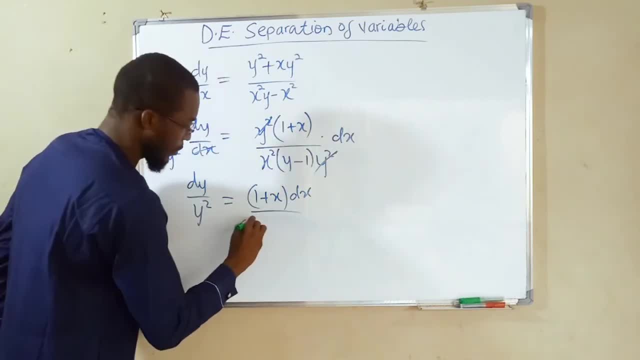 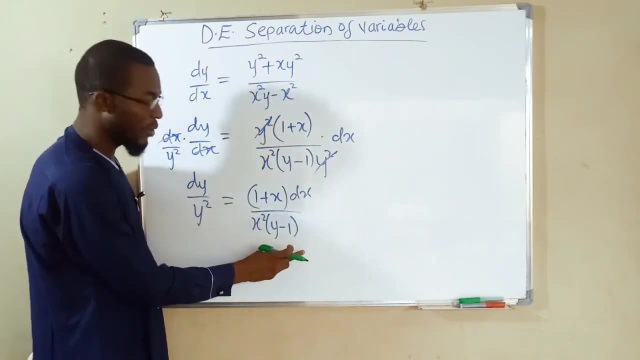 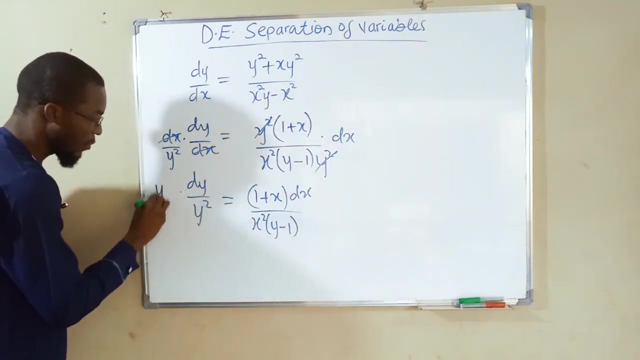 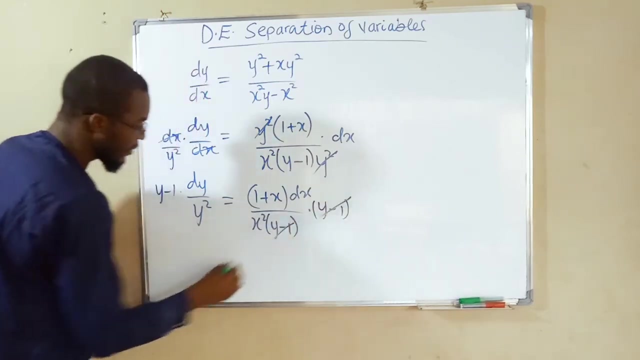 over x, squared y minus 1.. We still have y minus 1 to the right-hand side. Therefore, we are going to multiply by y minus 1.. So we have y minus 1 and y minus 1.. So that this will cancel this. 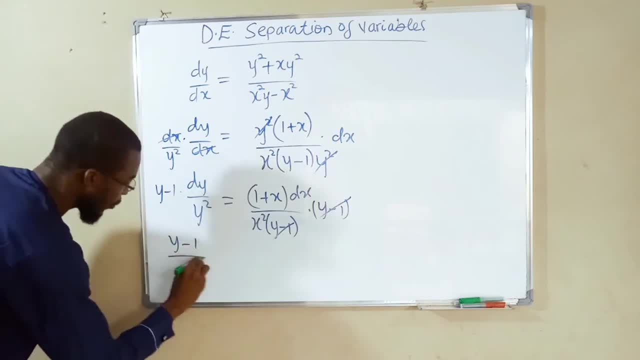 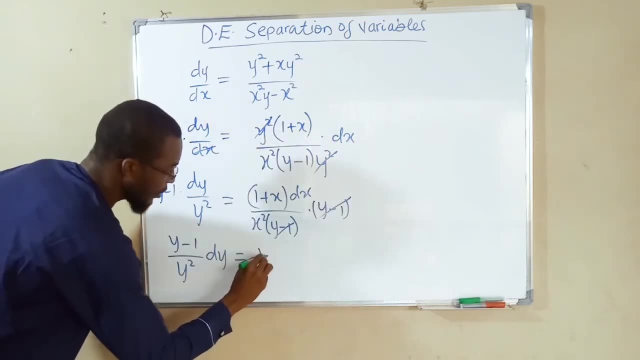 Finally, we have y minus 1 over y squared dy And to the right-hand side, we have 1 plus x over x squared dx. Let us do the same thing on the other side. Let us do the same thing on the other side. 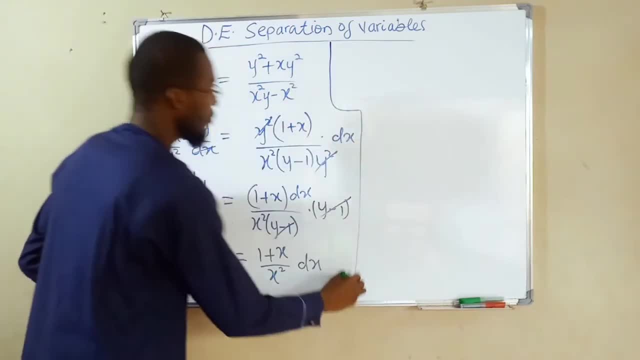 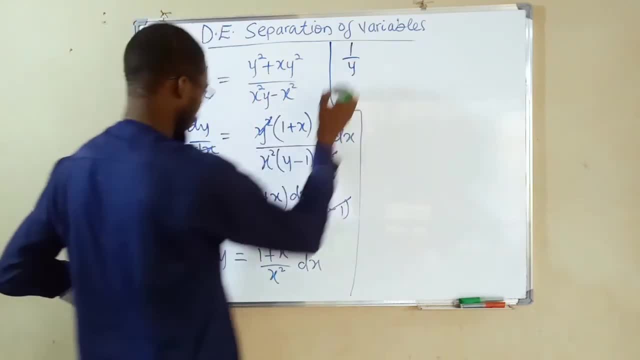 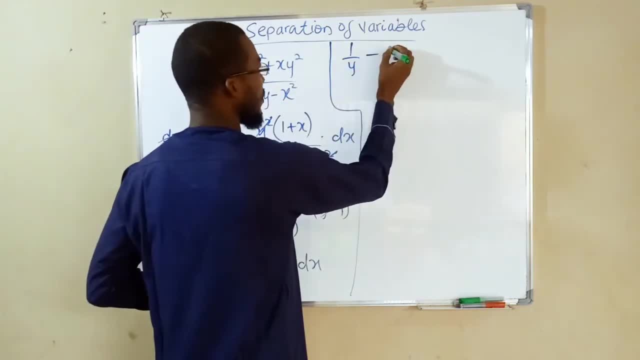 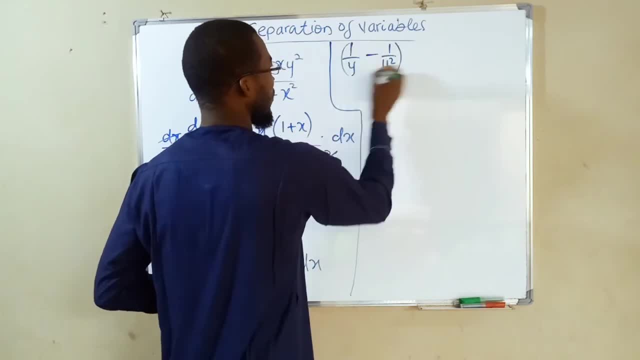 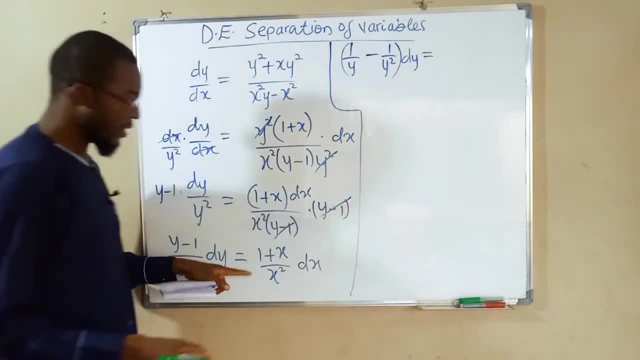 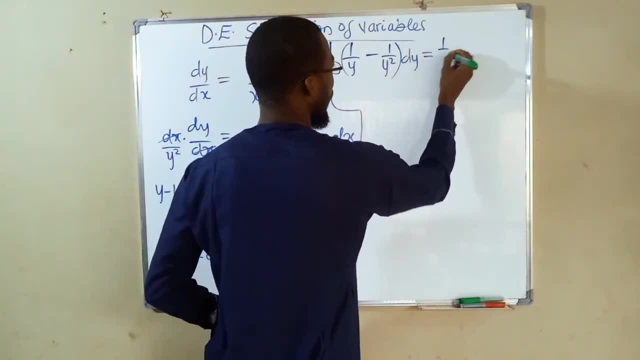 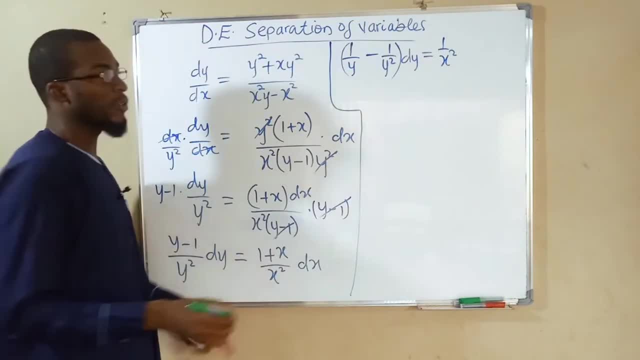 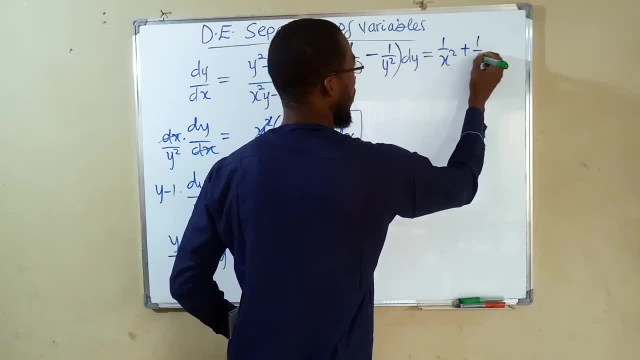 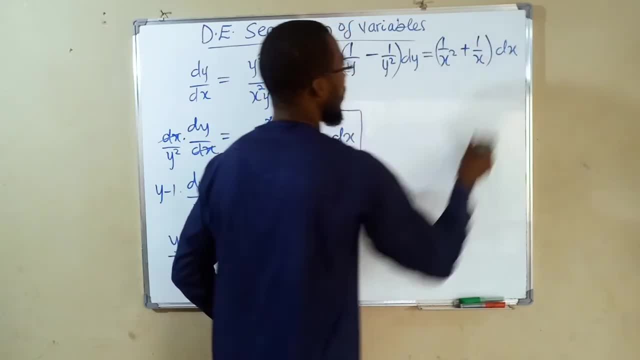 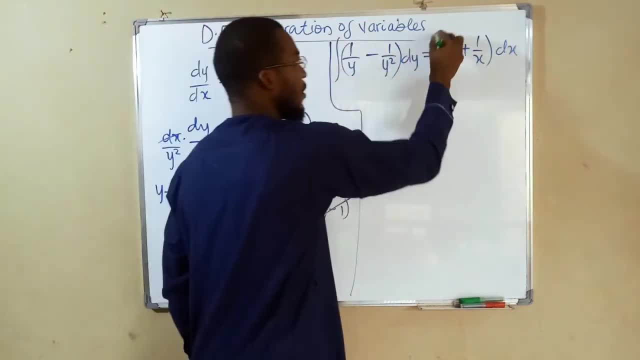 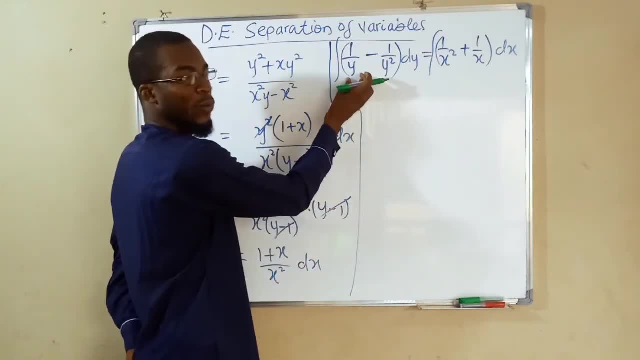 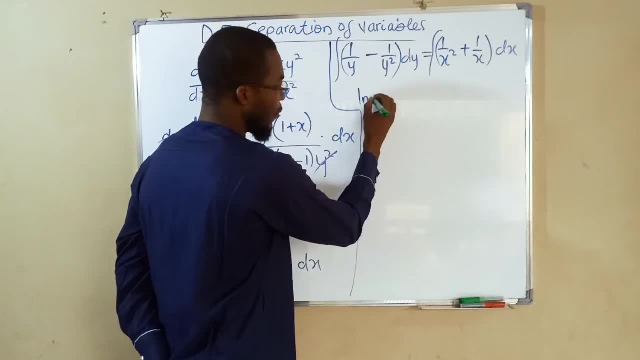 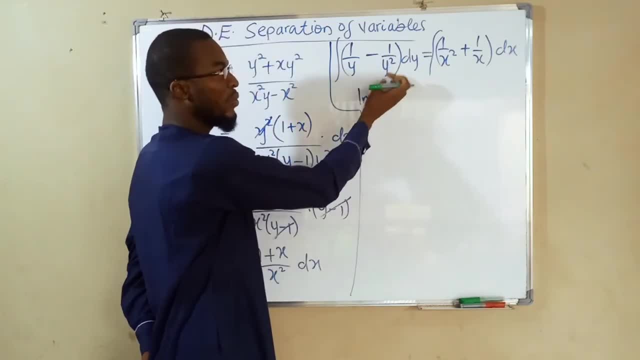 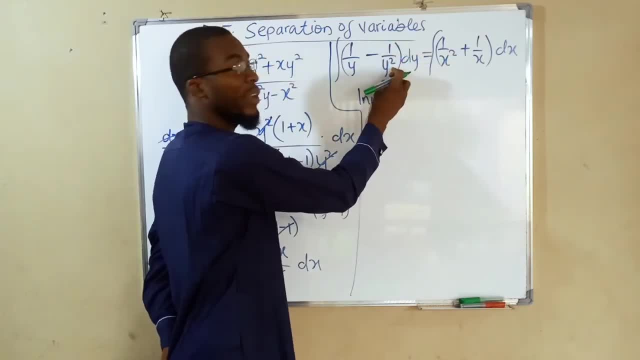 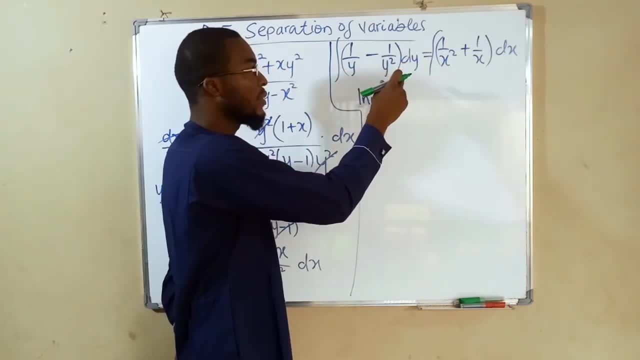 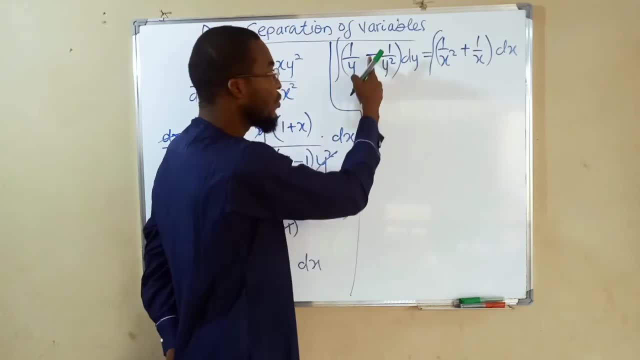 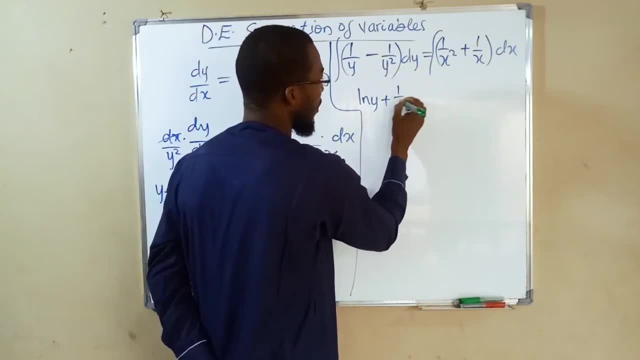 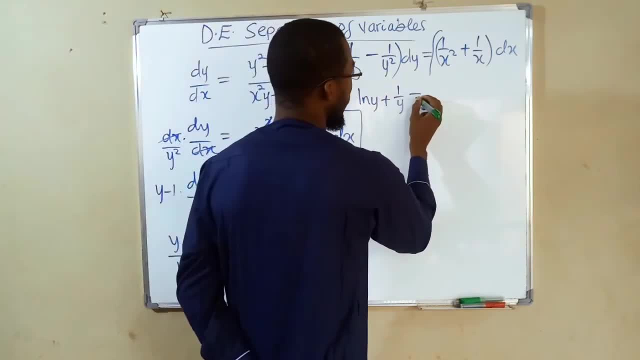 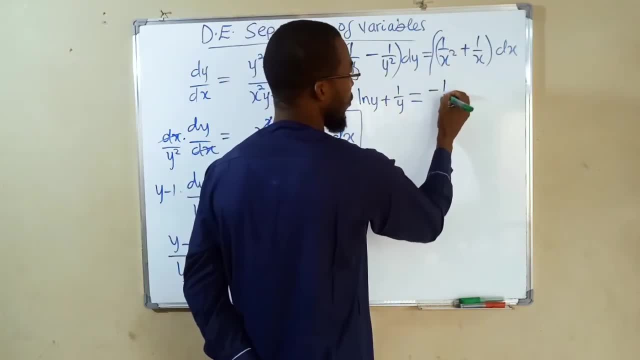 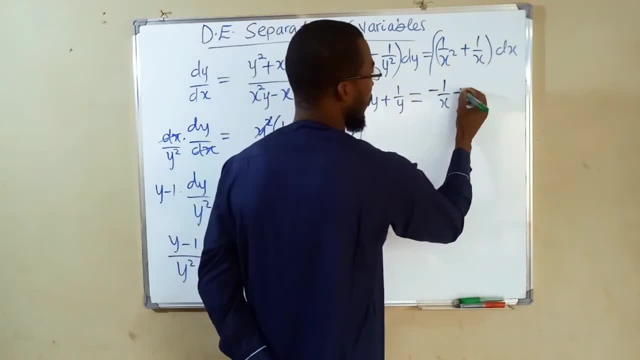 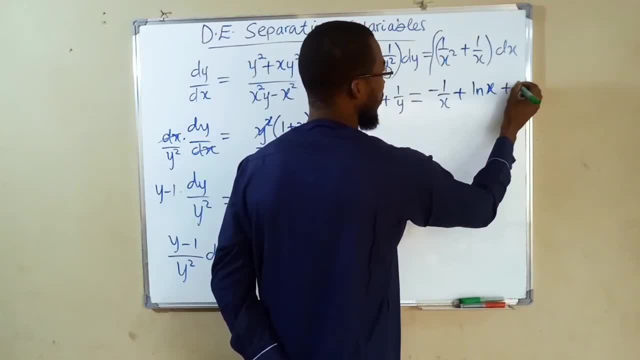 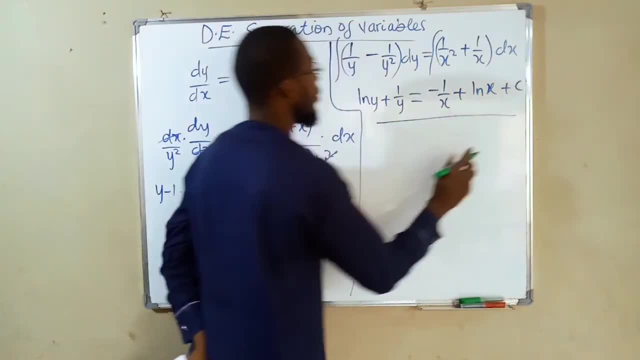 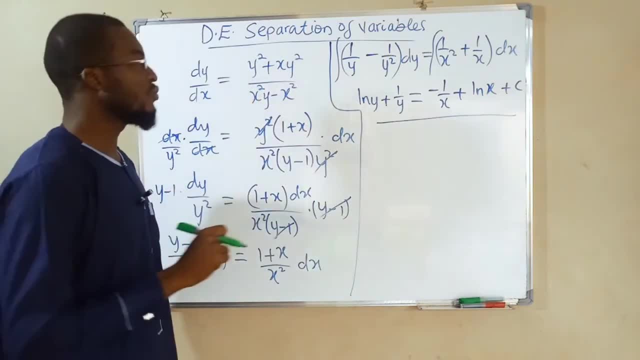 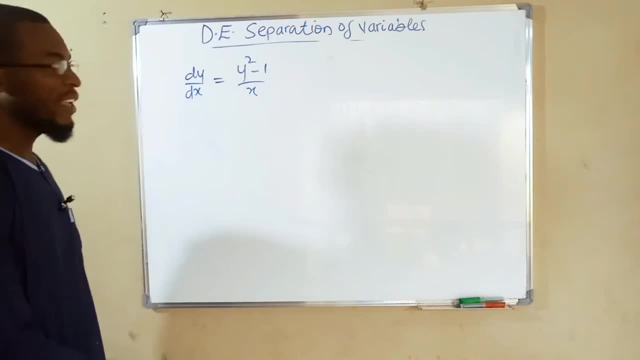 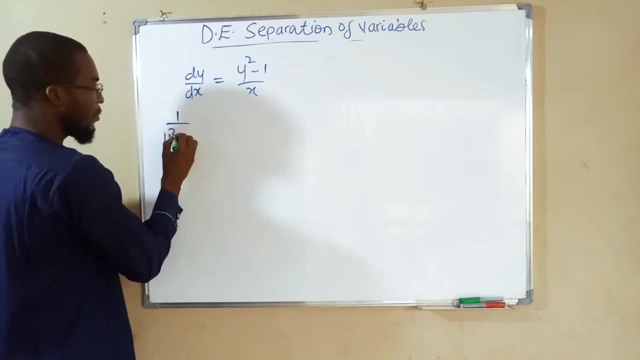 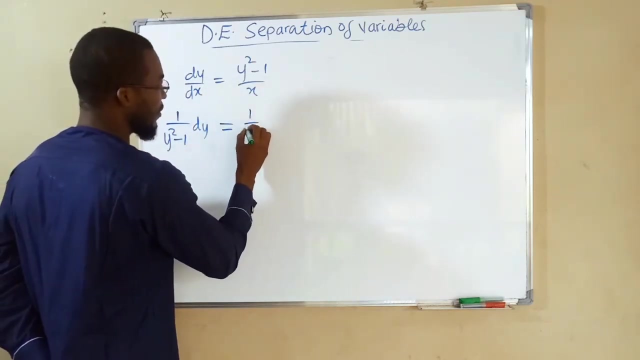 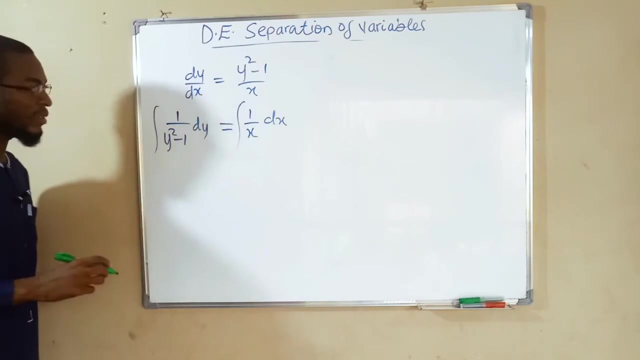 one. This is our next question. Again, we have to separate the variables. So we have 1 over y squared minus 1 dy to the left hand side and to the right hand side. we have 1 over x dx- Integrate this side, integrate the other side. But y squared minus 1 can be factorized. 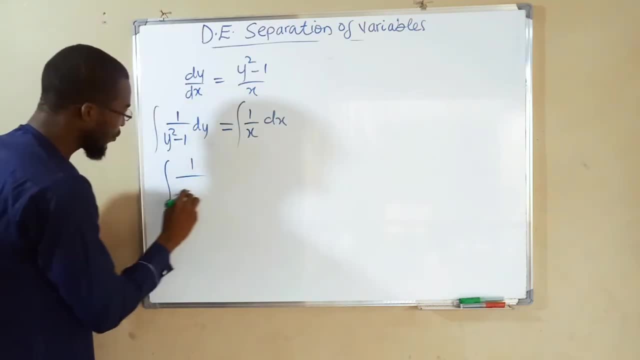 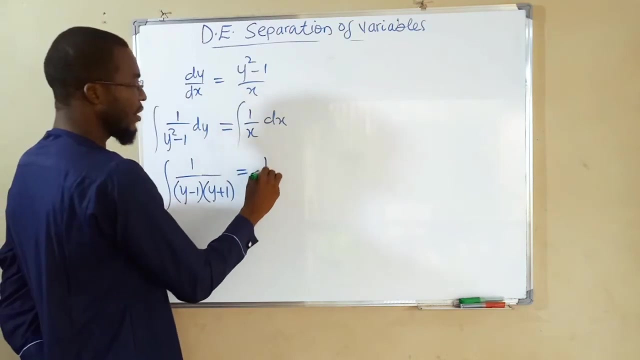 so we have which is a difference of two squares, is going to be y minus 1, y plus 1.. And to the other side we have the integral of 1 over x is just natural log of x. We are not done. 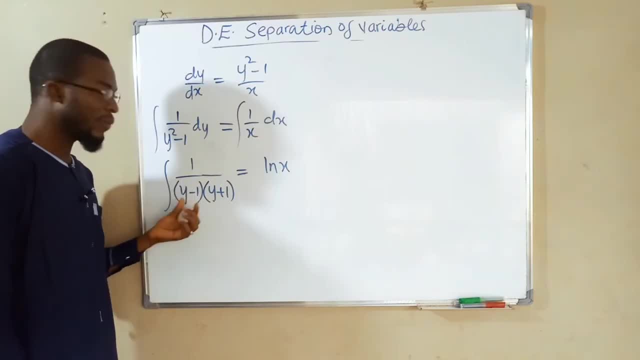 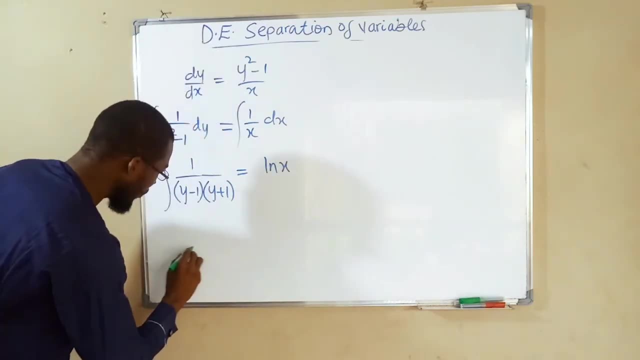 with this. yet To find the integral of 1 over this function, let us split this into a partial fraction. It is going to be 1 over x, dx, The integral of 2 times the first one is going to be y minus 1, then y plus 1.. Using: 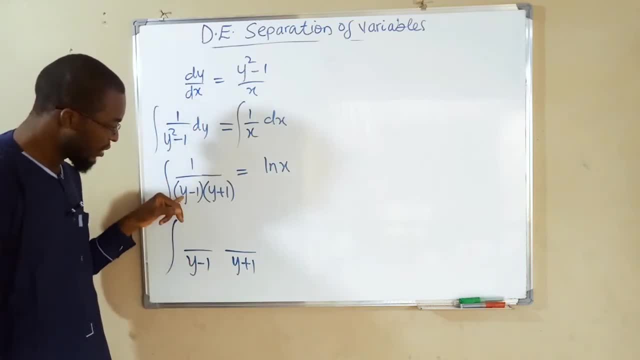 Cobb-Aub method. this is y minus 1, which is this: To transform y minus 1 into 0, y must be equal to 1, which is 1 minus 1 equal to 0. So we are going to substitute it here. 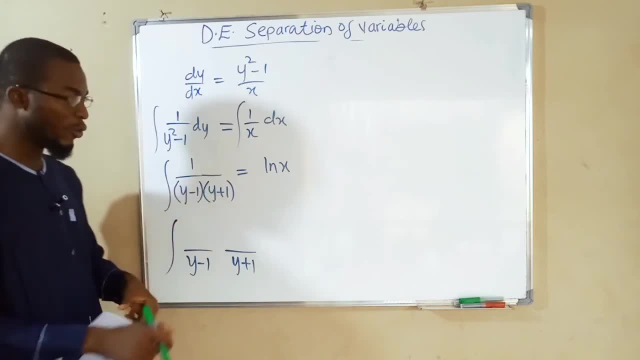 If y is 1, we have 1 plus 1.. 1 plus 1, which is equal to 2.. And here we have only 1, so we have 1, 2.. Then, to the other side, we have y plus 1, and this is our y plus 1.. To transform this into 0,, we have: 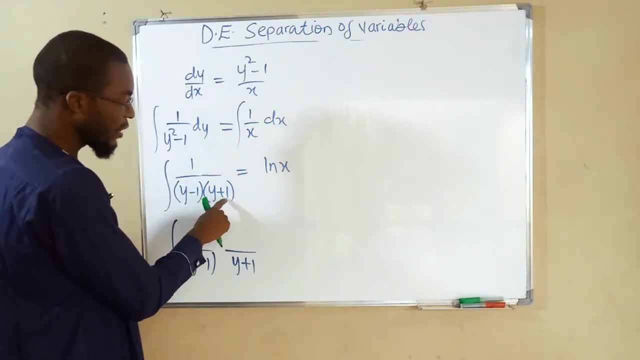 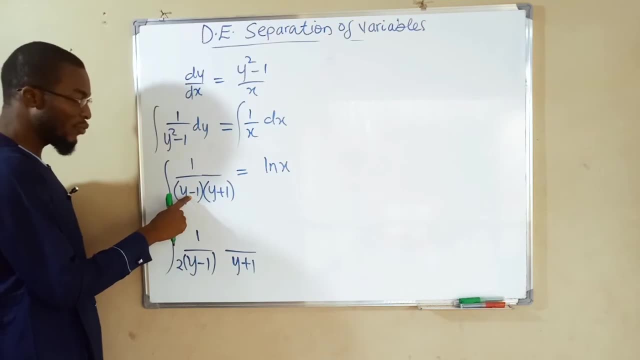 to set y to be equal to negative 1.. Negative 1 plus positive 1 is 0. So we are going to substitute it here: Negative 1, negative 1 is going to be negative 2.. So we have 1,, 2,. 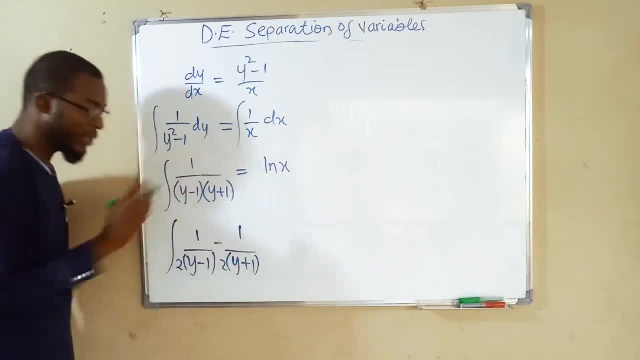 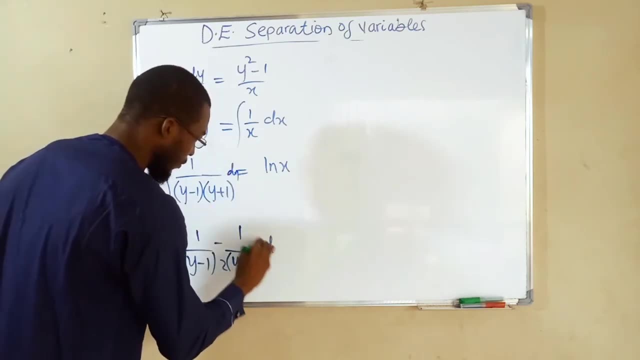 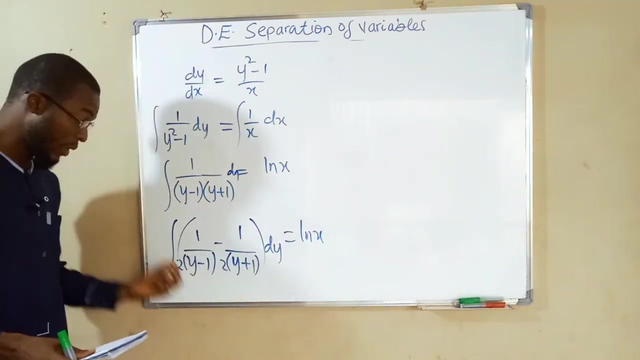 2, net 2 plus and y plus 1 is going to be negative, 1., Negative, 2.. So this is what we have to integrate with respect to dy, The whole of this with respect to dy, And this is equal to natural log of x. We are going to integrate them independently. 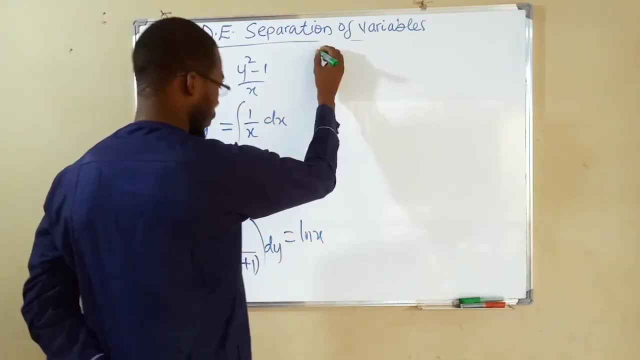 for this We have. if you integrate this, you are going to obtain 1 over 2.. Already, we have 1 over 2.. So what you are going to do here is you are going to get 1 over x. 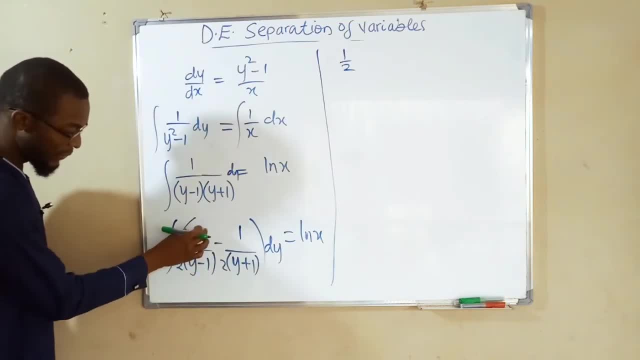 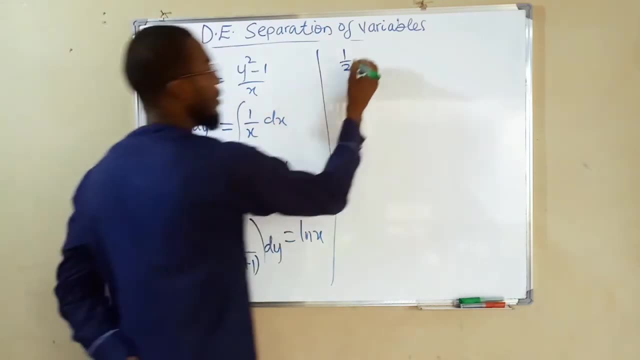 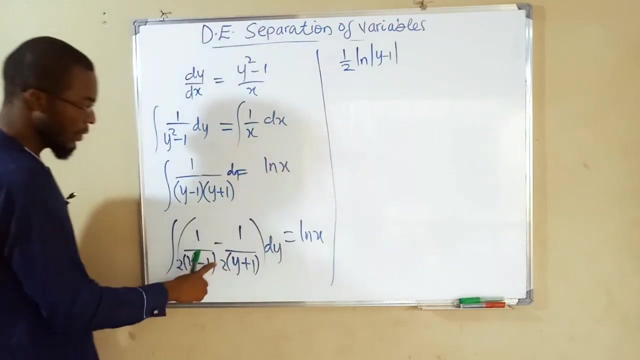 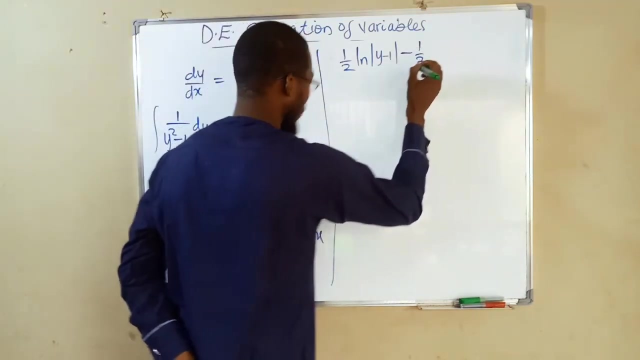 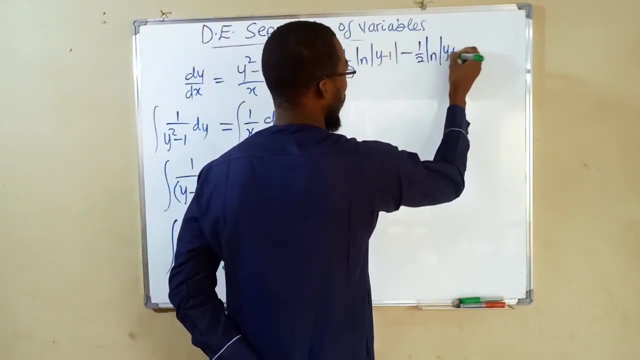 you can factor it out. then if you integrate 1 over y minus 1, you're going to obtain the natural log of y minus 1. so we have natural log of y minus 1, minus this one too. it has 1 over 2 as factored the natural log of y plus 1. and 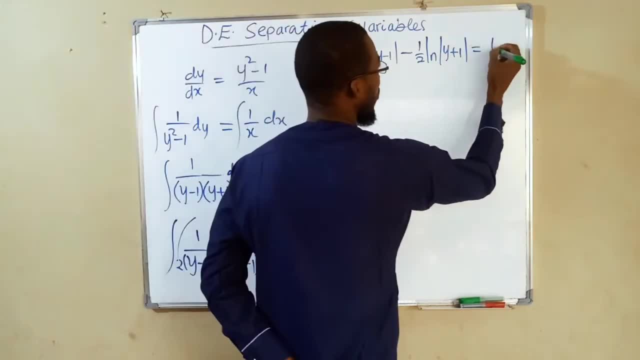 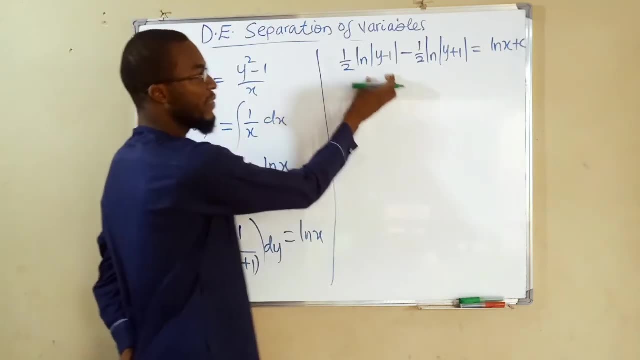 to the other side. we have natural log of X plus our constant of integration. this is our general solution. but if you want to get rid of the natural logs, you can do that by connecting the natural log of x to the natural log of y minus 1 and. 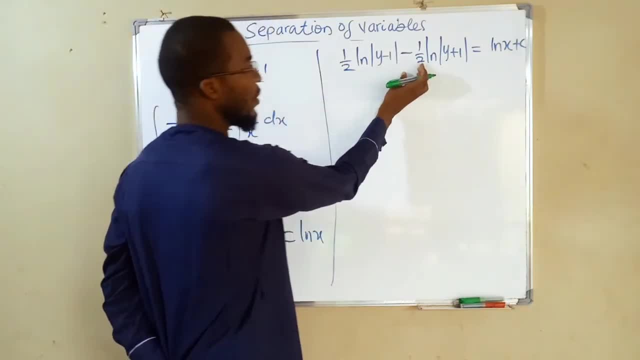 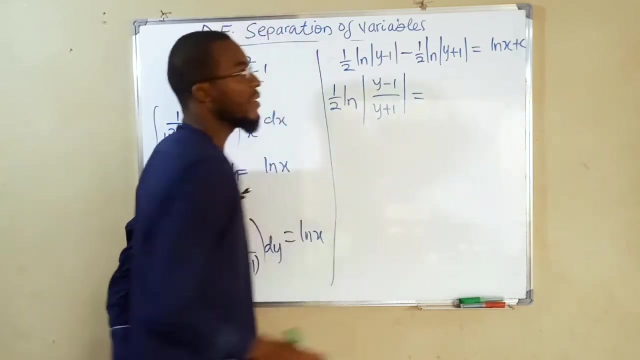 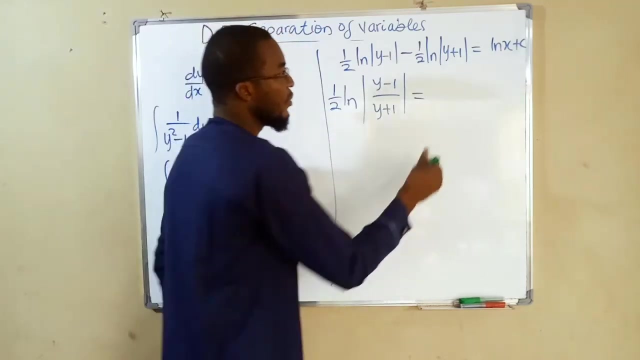 connecting the logs together. so we have one half in common. so we have 1 over 2. the natural log of y minus 1 divided by y plus 1, until the other side. if you set our constant to be a natural constant and connect the two together, you're going to obtain natural log of C X. 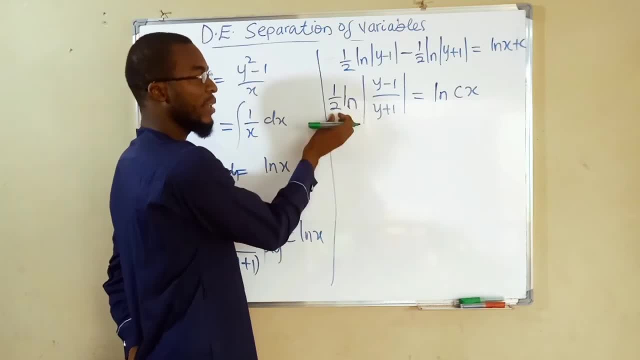 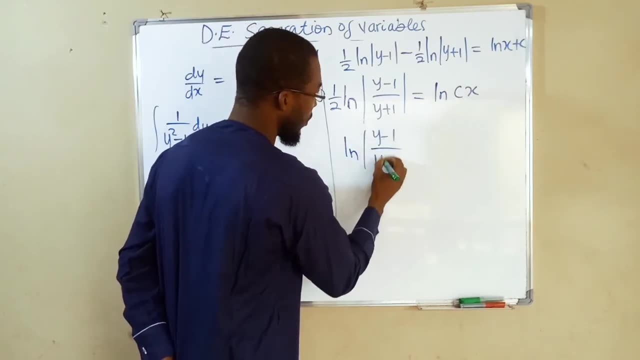 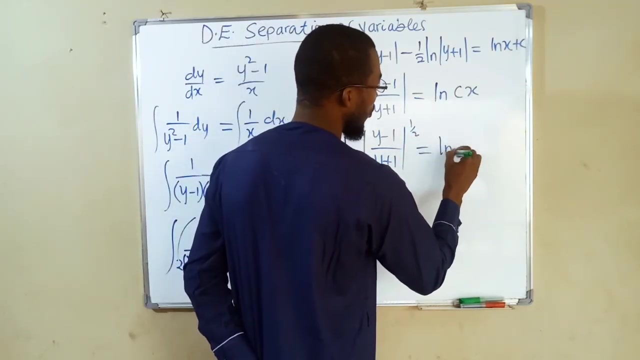 from the law of logarithms, and this time can take the power of half. so we have natural log of y minus 1 over y plus 1 to the power of 1 over 2. this is equal to the natural log of C- X. so what times have natural log in common? so they. 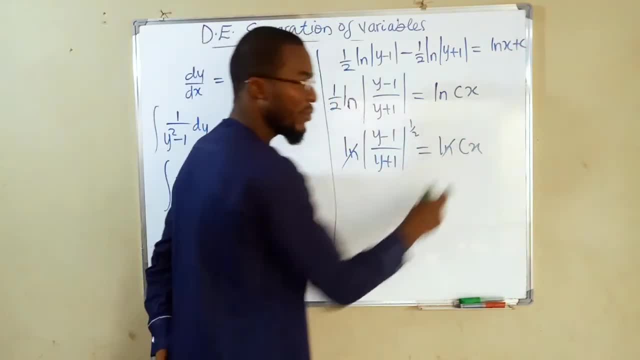 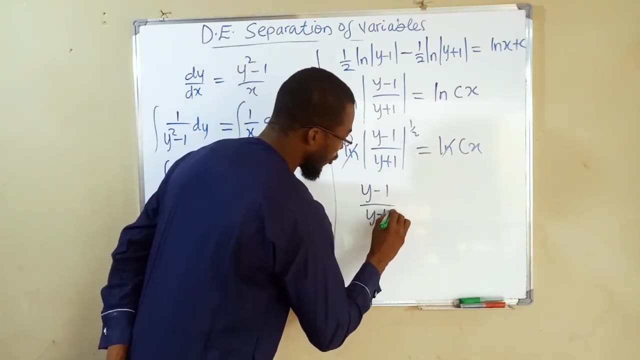 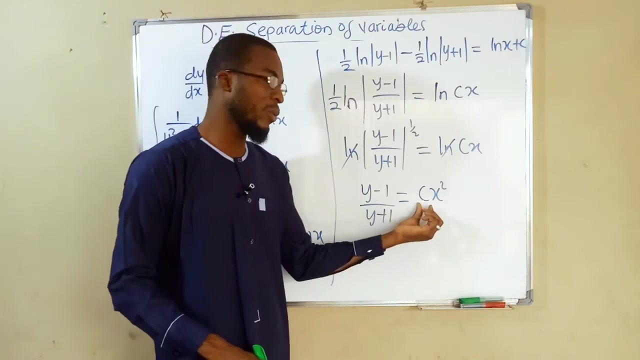 cancel out. but you can take this power to the right hand side, which is going to make it squared. so from the left hand side we have a constant of y minus 1 over y plus 1 and this is equal to C. X squared constant doesn't have to take the power because constant squared is still constant. you. 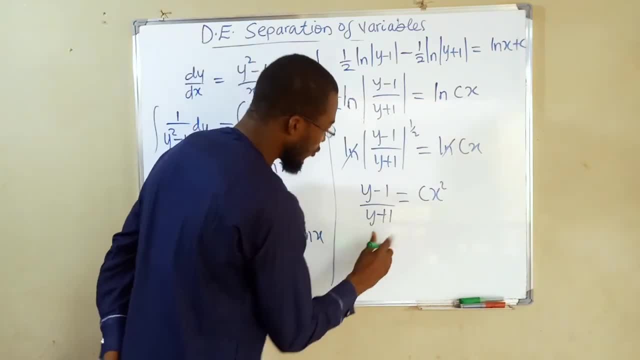 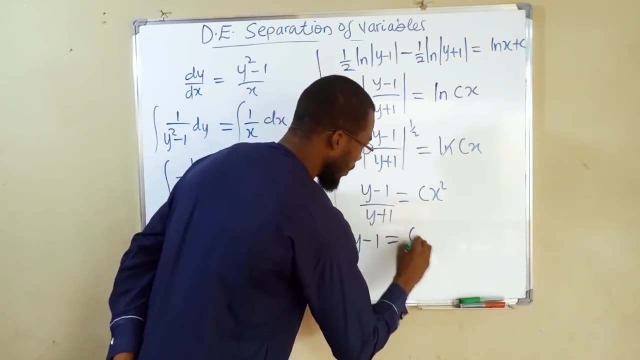 can even clear the fraction by multiplying both times by y plus 1. so we have, from the left hand side, y minus 1, and this is equal to C X squared times y plus 1. therefore, we have a constant of y minus 1 over y plus 1, and this is equal to C X squared times y plus 1. therefore, we have a. 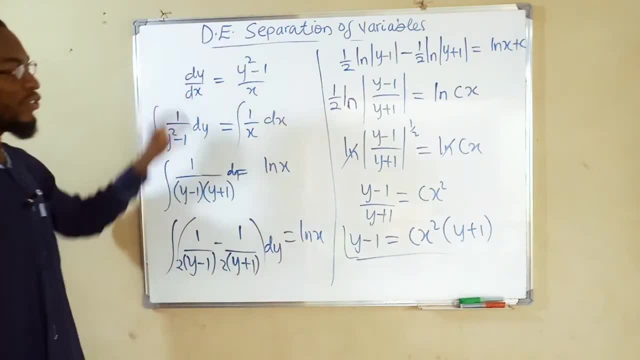 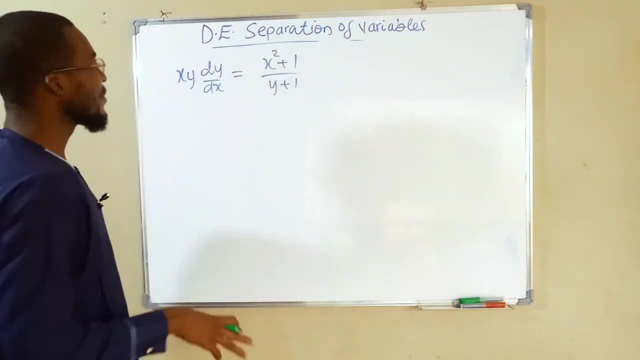 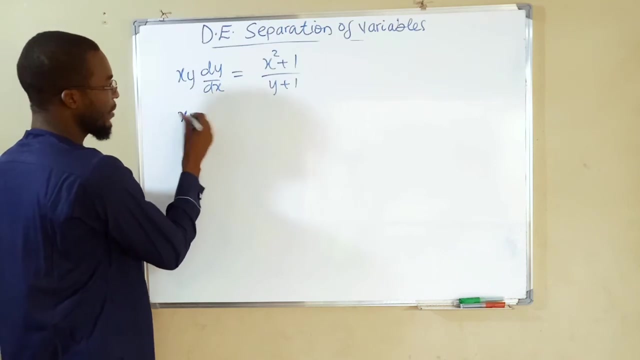 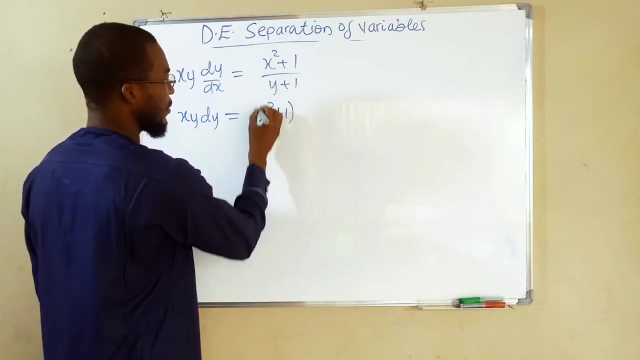 of 10, the general solution for this differential equation. so now let us look on to the next question. this is our next question again. first of all, let us take the x to the right hand side, so that we have x, y, dy, and to the other side we have x squared plus 1, dx over y plus 1. 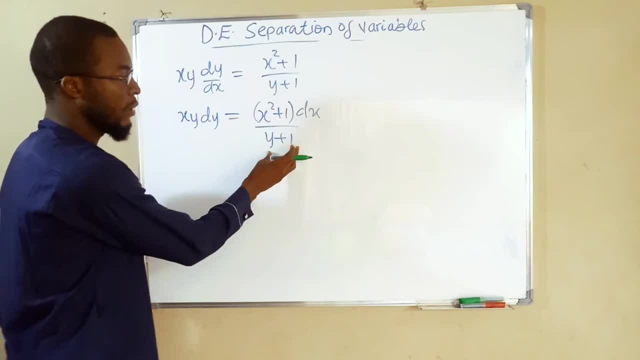 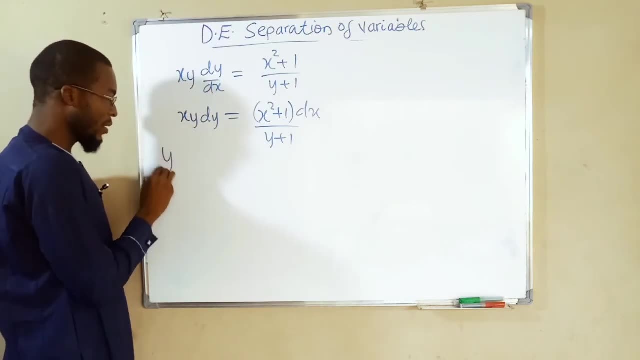 Now let us bring this from backward. if y plus 1 comes to the left hand side, it will multiply, and we have y here. so we have y times y plus 1, and we are taking x to the right hand side, but we still have dy here. this is equal to: if x crosses over, it will divide. 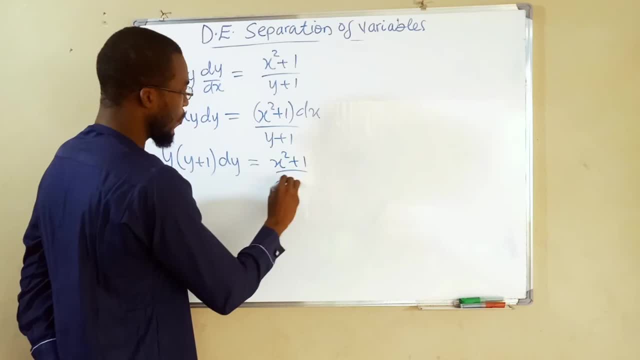 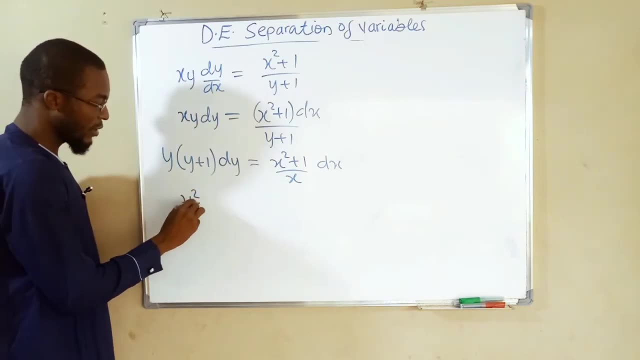 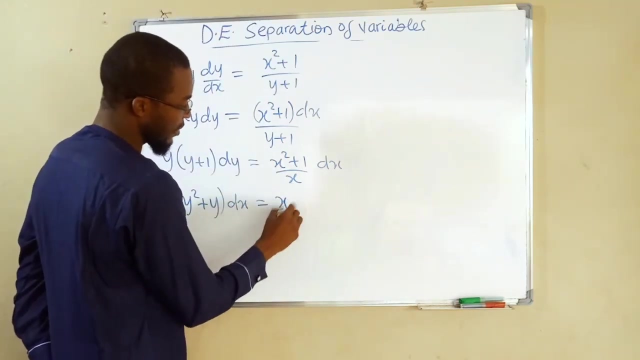 so we have x squared plus 1 over x, and this is our dx. Let us further simplify this time. this is going to make it y squared plus y, all dy, and this is equal to this. divided by this is x, and 1 divided by x is 1 over x, all dx. 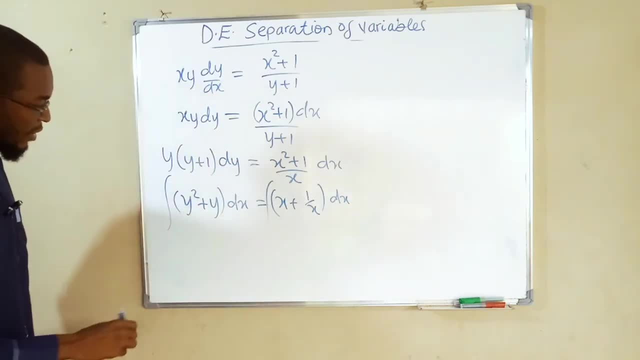 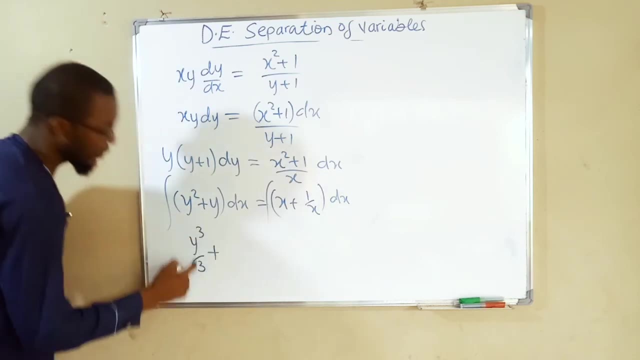 Now we are free to integrate both sides of this equation. For this we are going to have y to the power of 3 over 3, plus y squared plus y squared plus y squared Over 2, and this is equal to, to the right hand side we have. this is going to make it. 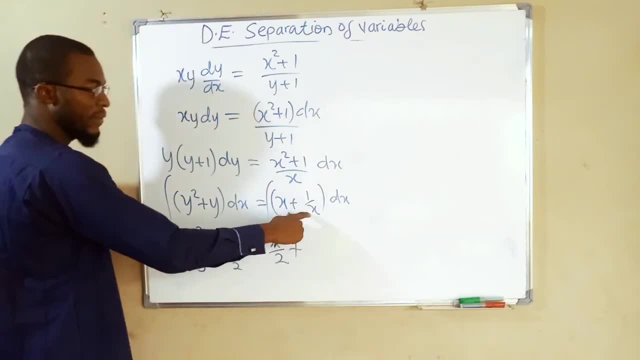 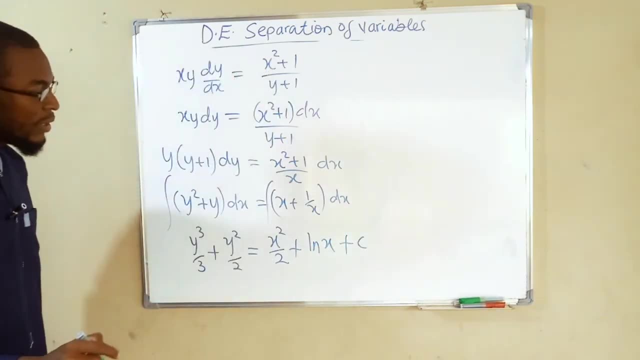 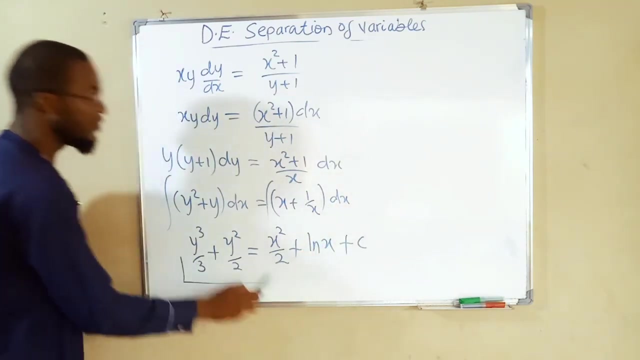 x squared over 2 plus. if you integrate this, you are going to obtain the natural log of x and plus our constant of integration. If you like, you can reduce the fraction. if you like, you can leave your answer this form. This is the general solution for this differential equation. 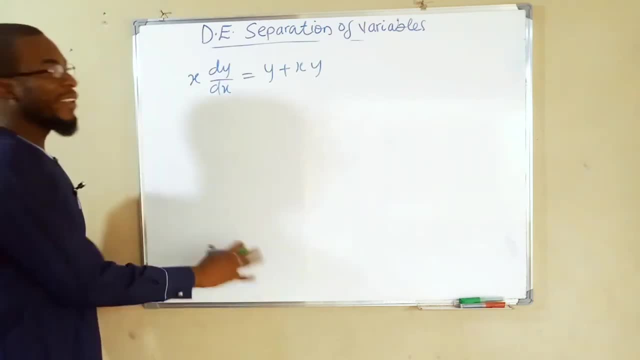 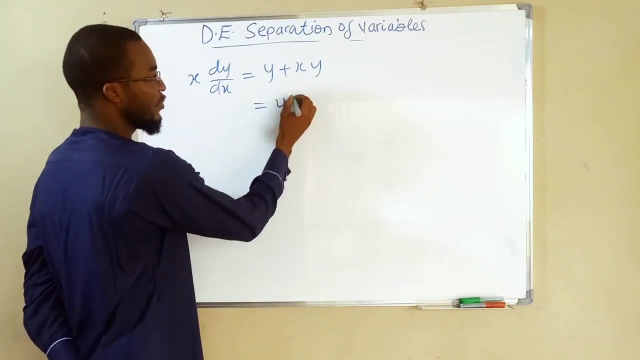 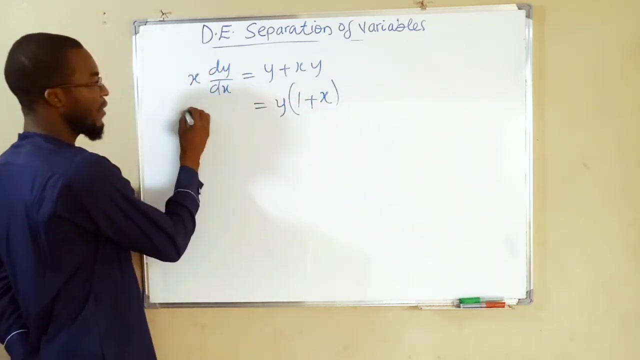 Now let us look on to the last question. All right, this is our last question for today. Again, let us factorize this side. so we have y in common. between the two terms first term remain 1 plus the second term remain x, and here we have x, dy over dx. 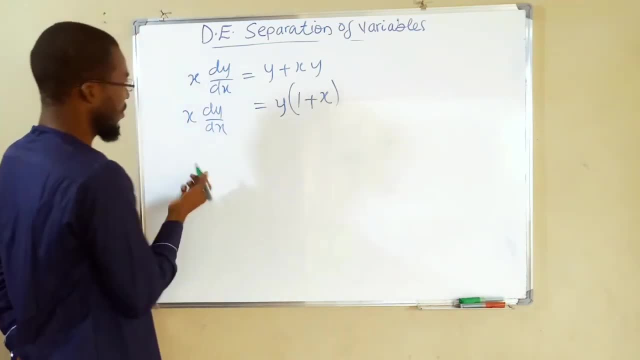 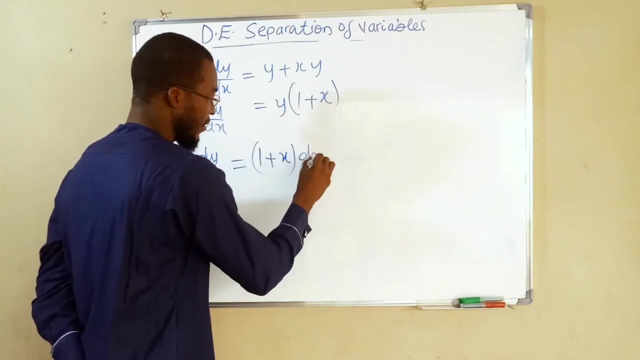 Again. let us take this dx to the other side and bring y to this side. so we have x divided by dy over y, because y is coming backward. it is multiplying here. therefore it is going to divide the other side. This is dividing here. it is going to multiply the other side. so we have 1 plus x dx. 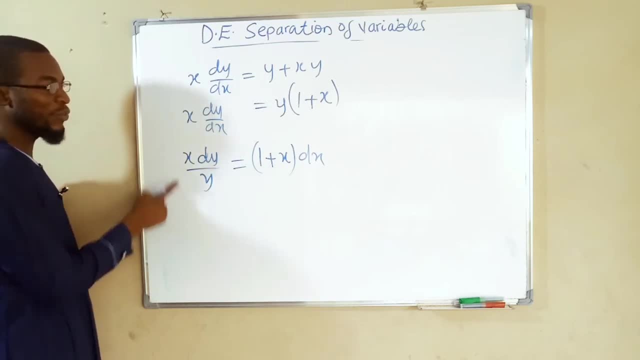 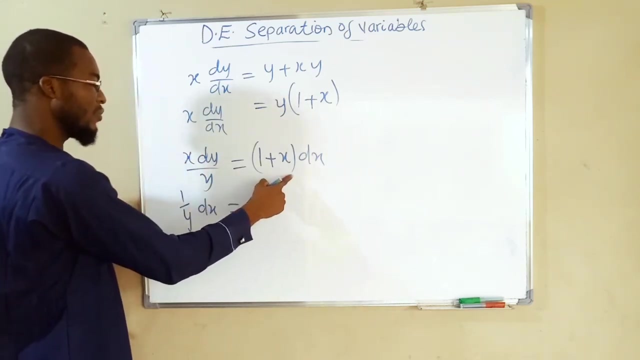 We still have x to the left hand side, which we are going to take over. so we have dy over. we say 1 over y, dy is all the same. This is equal to x is going to divide this term. let us do it directly. we have 1 over. 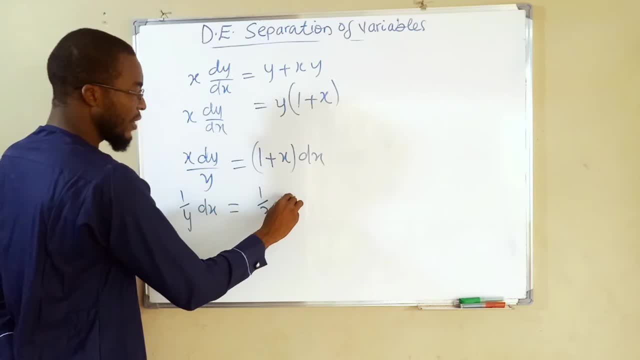 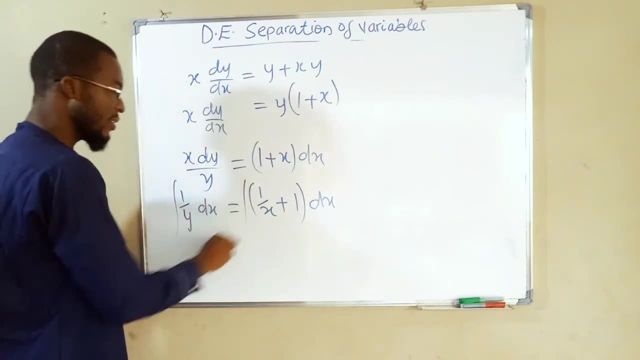 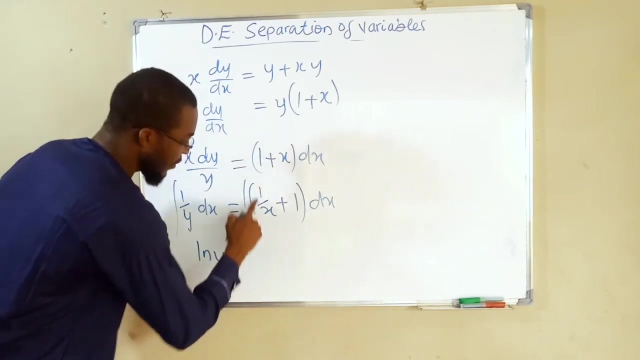 x plus x divided by x, is going to make it 1, all dx. Now we are free to integrate, integrating this side, integrating the other side. From here, we have natural log of y. this is equal to, this is the same term as natural. 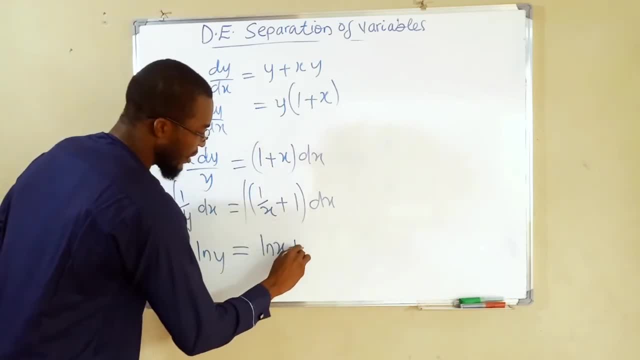 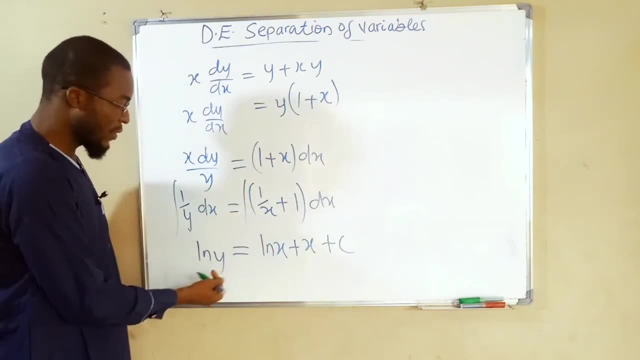 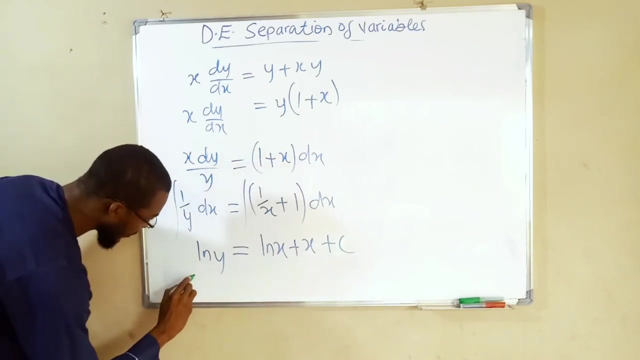 log of x, and this is going to be x, x plus constant of integration. This is enough to be our general solution, but if you like, you can manipulate this natural logarithm by bringing this one backward. we have natural log of y minus natural log of. 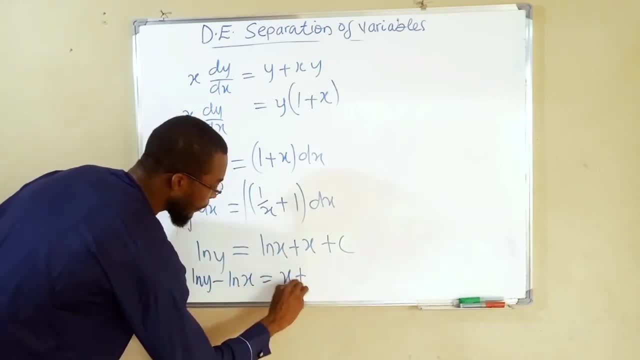 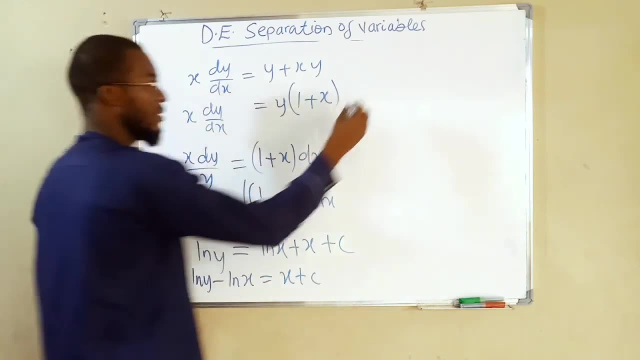 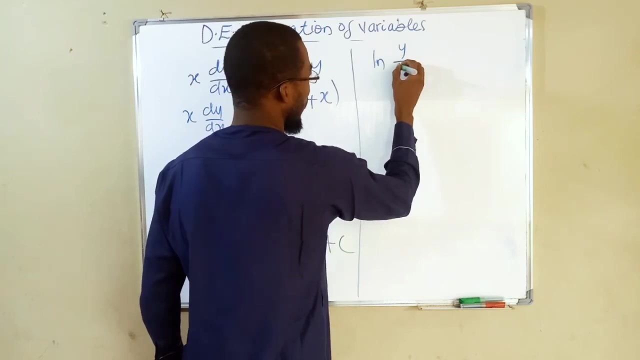 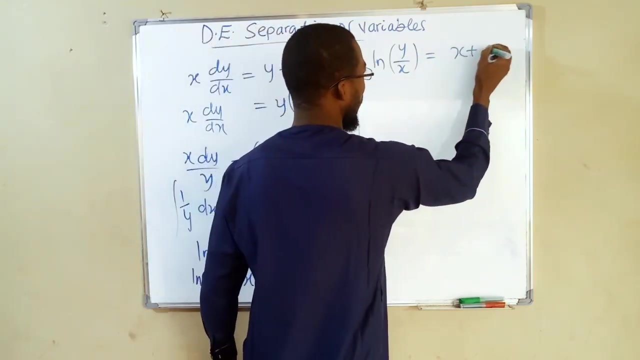 x And to the right hand side we have x plus c. These two terms have common log, so we can match the logs together so that our new log becomes natural log of y divided by x because of subtraction, And to the other side we have x plus c.